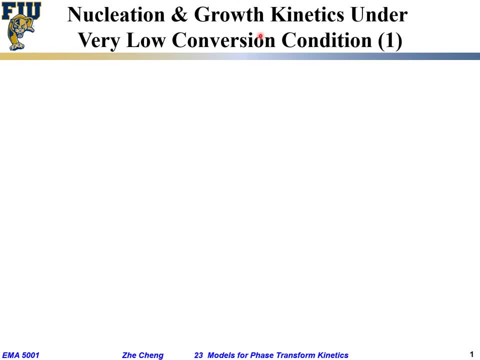 So now let's look at the simplest kinetic model, The simplest kinetic model that describes the extent of conversion under the very low conversion condition, which means when the reaction of its transformation just happened. how can we describe the extent of conversion with respect to time? That is what we call kinetics Relates: the extent of conversion. 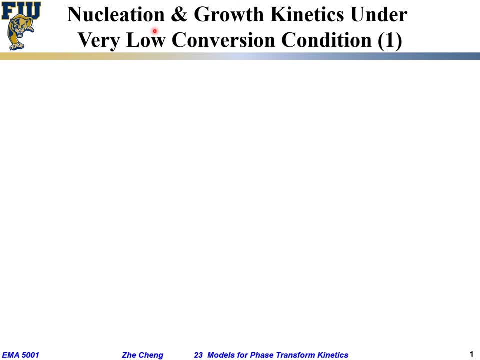 with reaction time, of its transformation time. Let's look at it So. let's say: this large circle represents the initial material and the wide portion represents so-called untransformed part within the material. And the small circles or spheres actually represent nuclei And the small 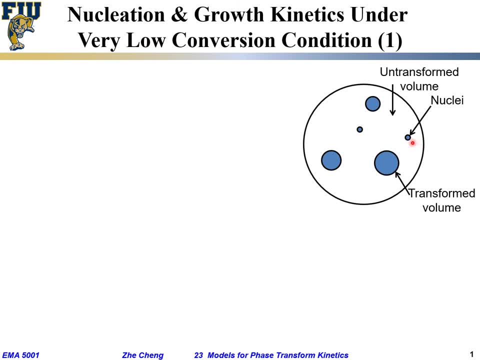 nuclei represent the initial material And the small nuclei represent the initial material And the nuclear. we put that in blue represents the different phase, let's say the precipitate phase, And some of the nuclei will grow larger into larger spheres and we call them transformed volume. 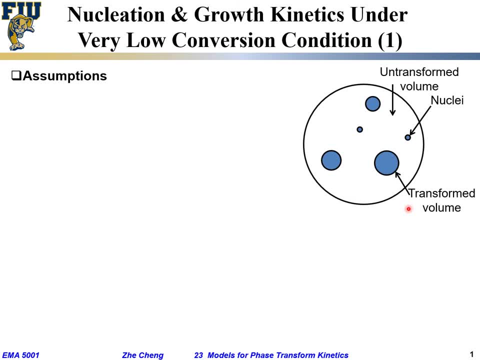 Okay, And to get this mathematical model to describe how fast that transformation happened with respect to time, we have to make certain assumptions. The first one, as we said, these types of nucleus- for simplicity, let's assume they are all spheres or spherical beta. 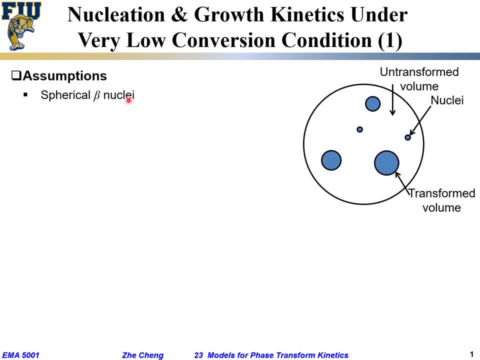 nuclei. Okay, Make sense, That's the simplest one that we can describe. And then let's, for simplicity, assume the nucleation rate is constant. value of N: Okay, Nucleation rate means per unit time, per unit volume of untransformed volume, how many new small nucleus form? 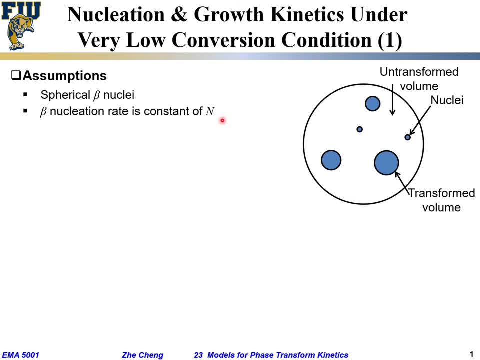 Okay, It has the unit of number per unit time, per unit volume. And then, for simplicity, let's also assume the linear growth rate of the nucleus radius, essentially di pleasures over dt, is constant of V. let's assume the radius grows linearly with respect to time. 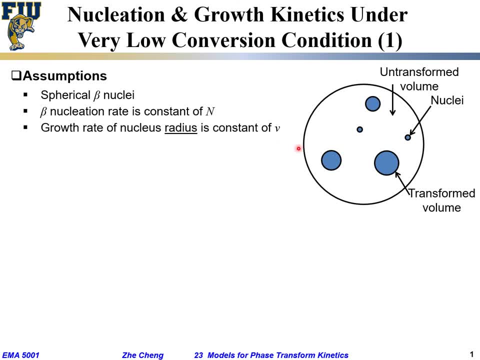 after it is formed with those assumptions and also assuming very low conversion with negligible overlapping. so we do not consider the case when one nuclear and another existing nuclear bump into each other or have overlap. that's for simplicity, over neglected. this is very true when, for so-called 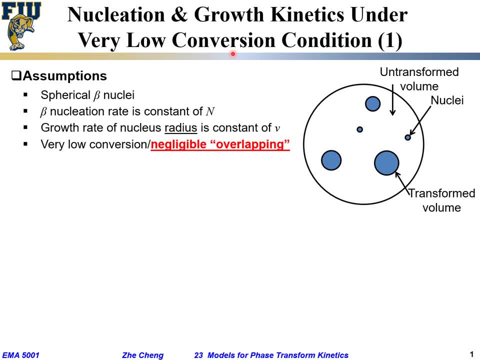 very low conversion condition, when the extent of reaction just happened, when the time t is very, very short. okay, with these assumptions, then let's say: at time t, at time t, the volume of single beta precipitate. a single beta precipitated nucleated formed at time tau would be this one. okay, we said the volume, okay, of a single beta precipitate. 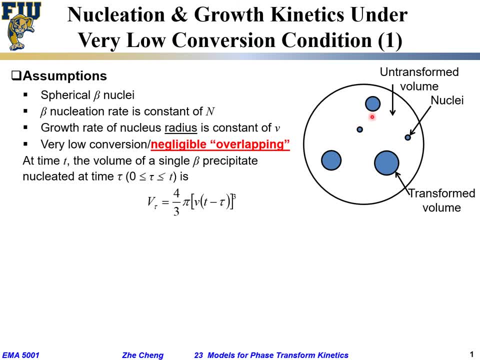 what shape is a precipitate? what shape are these precipitate? we said they are spheres, so that naturally the volume would be 4 over 3 pi. radius to the power of 3. okay, and then what is radius? radius, we remember, we said the radius is growing at a constant rate of V, but then the 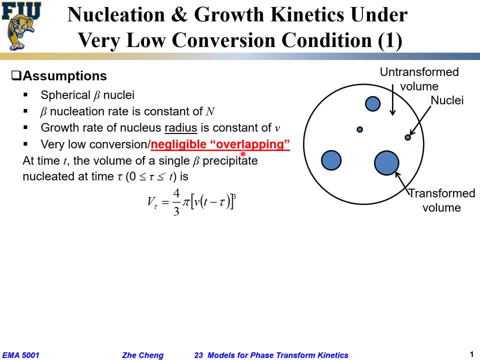 nucleus may form random form. it may not form at time 0, it may form at time tau and tau is greater than 0 but smaller than time t. okay, this is very important. we are considering at a time t the volume of a precipitate that spherical precipitate forms at time of. 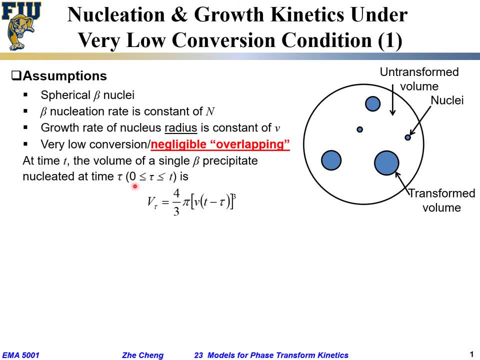 tau. it's formed not at the very beginning, not at t equals 0, but at tau, but tau is smaller than t. if tau equals to t, we assume the initial radius is essentially 0 but tau. if its tau is smaller than t, then at time t the total time for it left to grow. 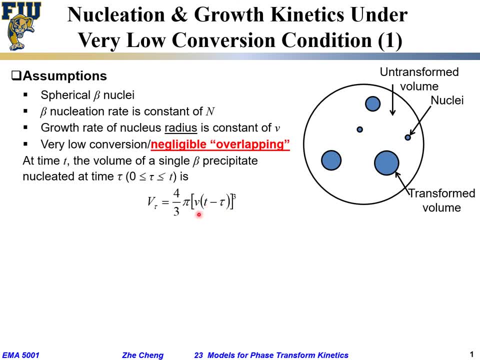 is t minus tau. okay, V times t minus tau gives it the radius of course we are assuming the initial nuclear size is negligible in it starts from 0 radius, which is a another assumption, our approximation. so this equation gives us the volume for a single spherical beta precipitate that formed at a time tau and then at time t, which is longer than tau. let's 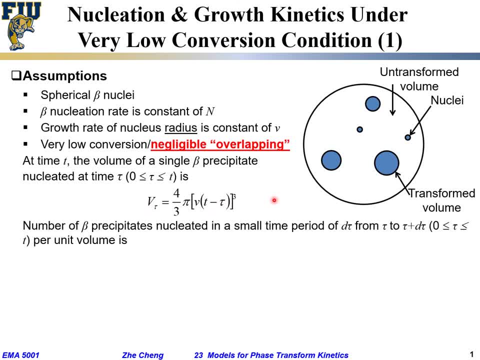 check what's the total volume, okay, and then the number. let's consider that's for one nuclear. what's the volume? and then let's consider what's the number of nucleus that are formed, the number of beta precipitated nucleated in a small time period, of d tau, of d tau. d tau means a incremental time. 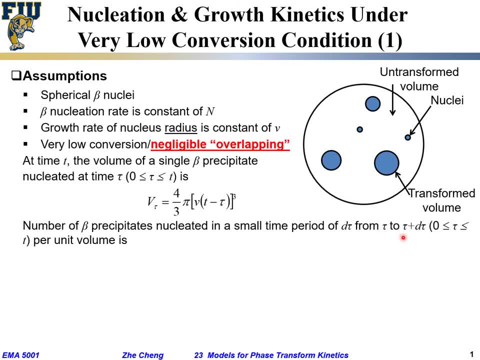 but d tau is from tau to tau plus d tau. tau is a time point and the tau plus d tau is another time point, which is slightly later than time t, so we are assuming the same thing. so we will see it later in the video than tau. how much later d tau? okay, it's d tau is our small incremental time, okay, and the number of? 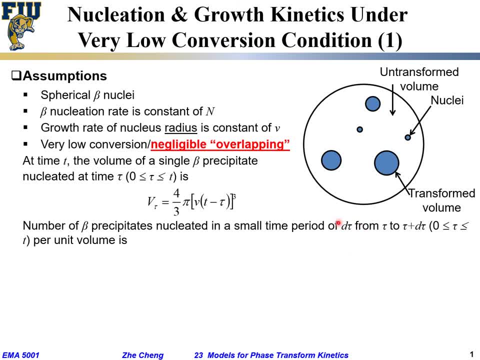 such spherical beta precipitate formed in that small incremental time of d tau per unit volume would be. we call it dn. dn equals n, which is our so-called constant nucleation rate, times, time, and of course we say per unit volume, so we can times one which is the same same value. so 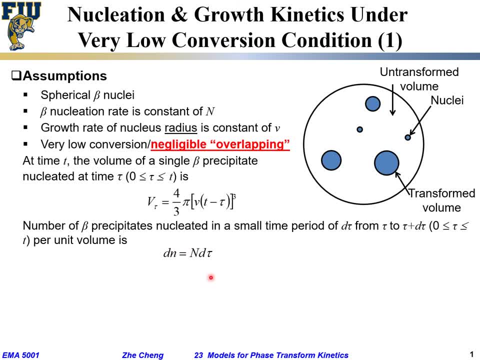 this equation, dn tells us the incremental, or the number of new beta precipitates created in the small incremental time of d tau, and then that d tau is from tau to tau plus d tau. okay, this equation gives us the number of new nucleus formed with these two. now we can calculate. 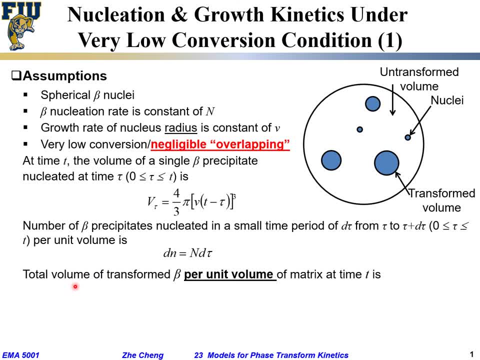 the total volume of transformed beta precipitate per unit. volume of the matrix at time t. now, at the time so-called t, which is of course, as we said, longer than at time t, the total volume would be a integration of the volume for each of the precipitate times. how many of the spherical precipitates 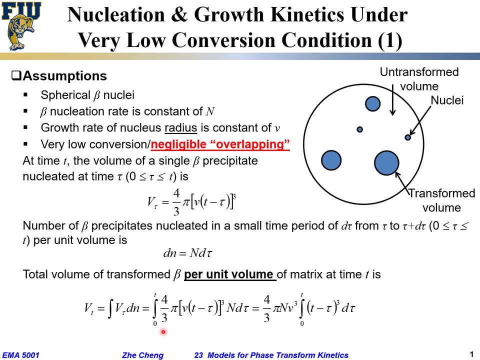 that are formed, okay. and then you, we do this integration from with respect to d tau. from here to here, we replaced the v? tau with pi over 3 times 4 vt minus tau to the power of 3, and then we replaced dn with capital: n times d tau. okay. 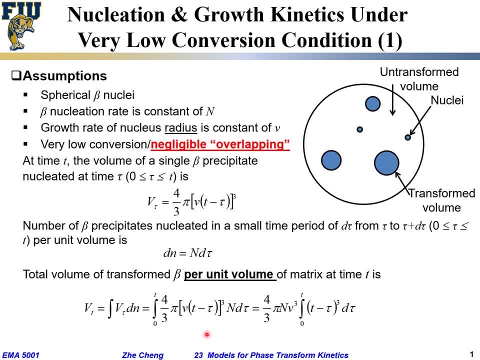 so that's for, from the first to the second again, the total volume of what the volume of the blue precipitates would be. integration means summation, summation of what summation of each of the precipitate it has this volume and how many of the precipitate. that's dn, and then we have to do this integration again. and within the bool, the total volume of precipitate is dn, and here we have to do this integration. Essence 10 will disappear. aspect and sabes. integration, volumization, Priest, desc, how, the volume of the precipitate, how many of the precipitate, that's the end. and then we have to do this integration, and here we have to do this integration of dn, and then we have to do this integration of this volume. our group, the DC and D and IV will be the integral of T, and so DC will not be discrete. for Do you want to solve that s of Kern French� dumb square? yet is it calledzos? just say: take it to August e, growing as, but basically, instead of 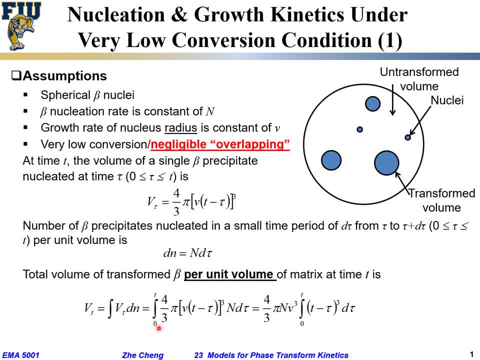 integration when the nucleus formed from time zero all the way to close to time t. that's this one. and then, of course, for this integration, you put four over three in outside of the integration symbol, pi, of course. take it out. n, let's assume, is constant nucleation rate. n can also be taken out. 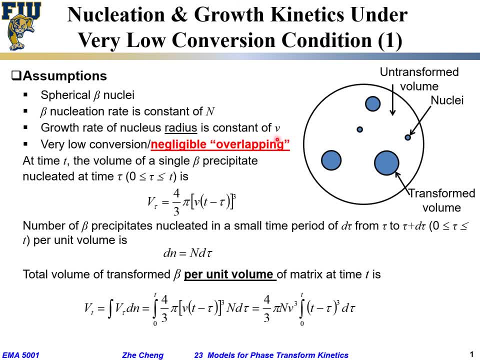 and we said constant growth rate. velocity can also be taken out, so the total volume of the beta precipitate at time. t per unit matrix volume would be four over three pi n v to the power of three times a integration term. okay again, n is so-called constant nucleation rate per unit volume. 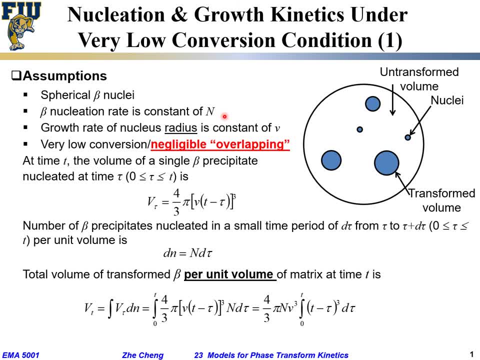 per unit time, per unit volume, how many new nucleus? spherical nucleus form. v is the so-called the linear growth rate of the nucleus. pay attention, radius. we are assuming that each of the nucleus is a sphere and the linear growth rate of the radius dr over dt. is this v and we said is a constant. 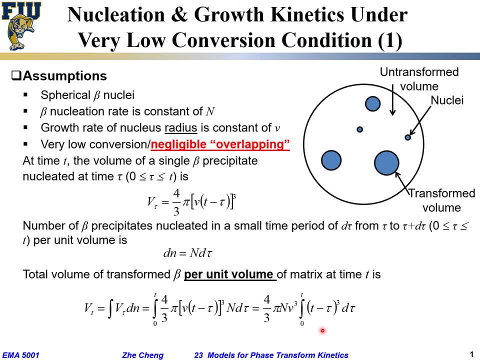 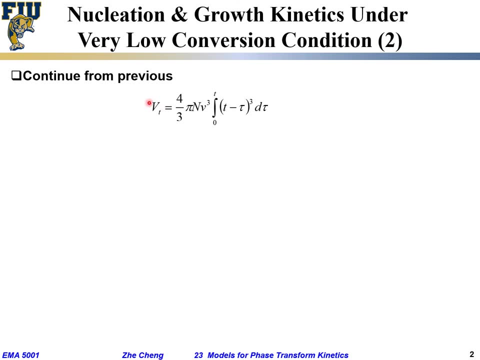 so we put this outside and then we are left with a integration term from zero point zero to t, t minus tau to the power of three d tau. okay, this is what we have: the total volume at time t for all those spherical precipidade that formed from time zero to time t. remember, the nucleation is random. the nucleation happens throughout from. 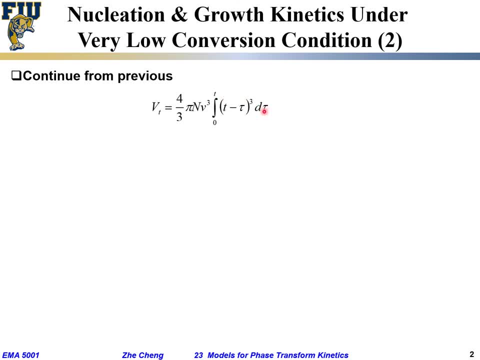 and each of the nucleus formed at a tau, it grows to certain size which is determined by the t minus tau to the power of three. okay, and if we do integration very simple- it's a fixed integration- we are going to get this one one over three pi, of course, constant n is, constant V to the power of three is: 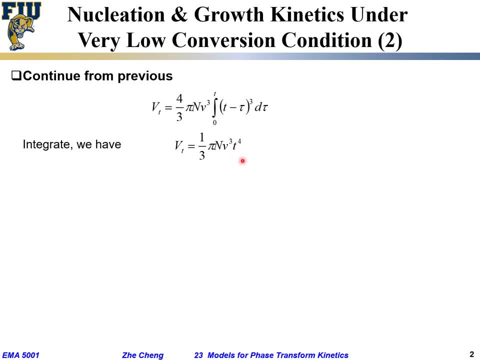 constant, but this term, integration term, becomes T to the power of force, from zero to T if we do this integration okay. so this equation: tell us the total volume of the precipitate and then, if our starting matrix phase is has unit volume, then the fraction of the 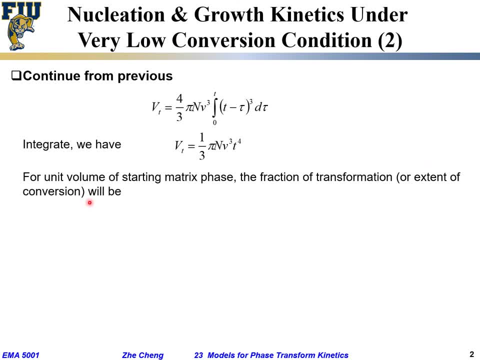 of transformation, or so-called extent of conversion, will be- I wrote it here- f. if that fraction of conversion, I call it f, will be the total volume of new precipitate divided by one, one for the unit volume of the starting matrix phase. of course V, T over one is just the same, which is one over three pi n V, three T to the power four. 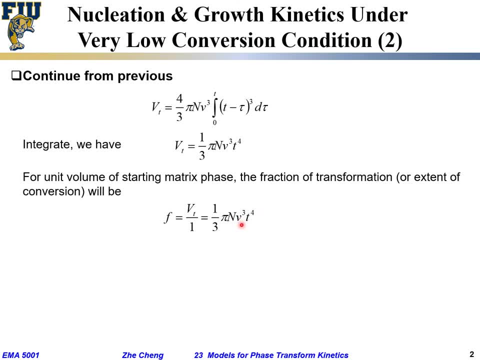 plus one over three pi n V. three T plus one over three pi n V. four again: n is nucleation rate. we said it's random but is a constant nucleation rate. V is the linear growth rate of the nucleus precipitated radius and the T would be. 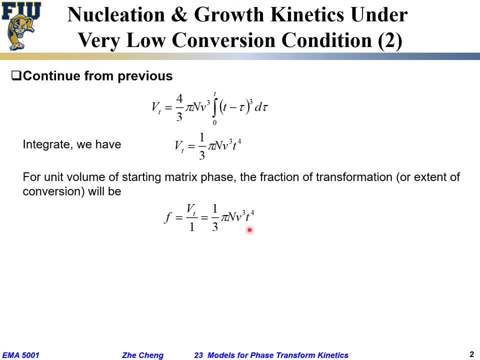 the time D. okay, and of course from this equation you see that the volume fraction would be higher if the time is longer, which makes sense- if the V growth rate would be faster than the intensification of the nucleus threshold, which makes sense if the V growth rate would be faster than the intensification of the nucleus threshold. 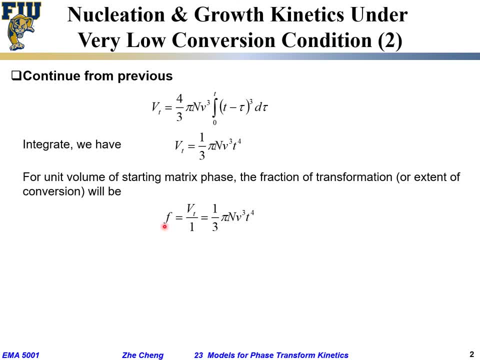 faster also makes sense. and also f would be- the fraction of conversion would be higher if n nucleation rate would be higher. and that makes total sense when you consider it okay. so we have a so-called simplest kinetic model that relates f the fraction of conversion. we're going 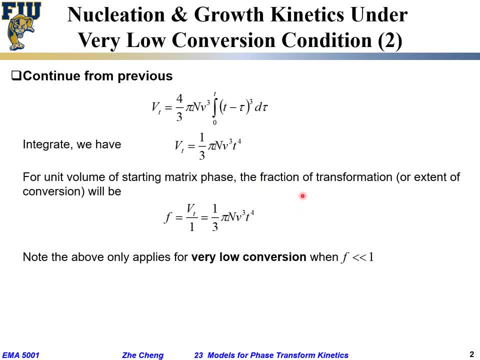 to refer to this concept a lot. the fraction of conversion, which means out of the matrix phase, what's the percentage? what's the fraction that got converted into the new phase which we call precipitate, for precipitation type of phase transformation. relates that with time, t and, of course, with other factors that are part of our model, part of our assumption. 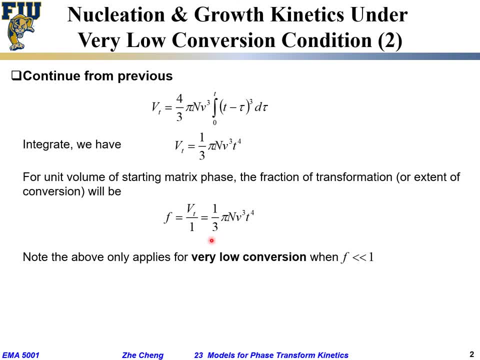 and one note about this equation is that it only applies for- read to yourself: very low extent of conversion. very low extent of conversion when this f value is much, much smaller than one. how small? let's say it's 0.01 or one percent or 0.05 or five percent. okay, higher than.